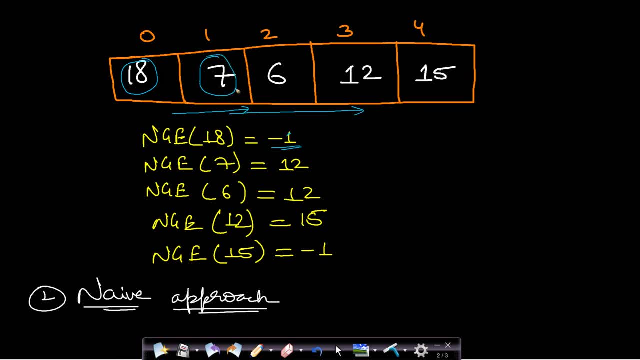 next greater element of this, 7?. The next greater element, that is, the closest element to the 7 which is lying to the right hand side and is greater than 7.. So the closest element to 7 which is greater than 7 is this: 12.. So the next greater element of this 7 will be 12.. Now the 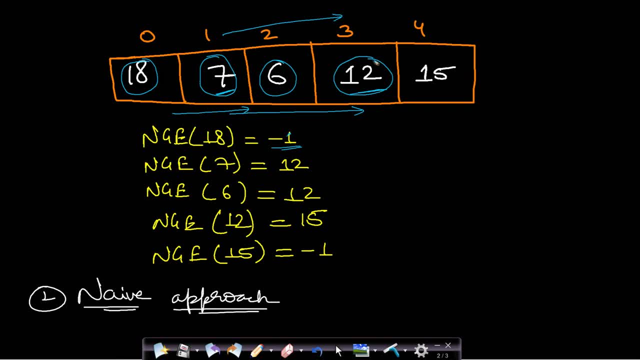 greater element of 6 will also be 12, and the next greater element of this 12 will be 15, and since this 15 is lying to the rightmost side, there will be no element to the right hand side, and so there will be no next greater element for this last element, and so 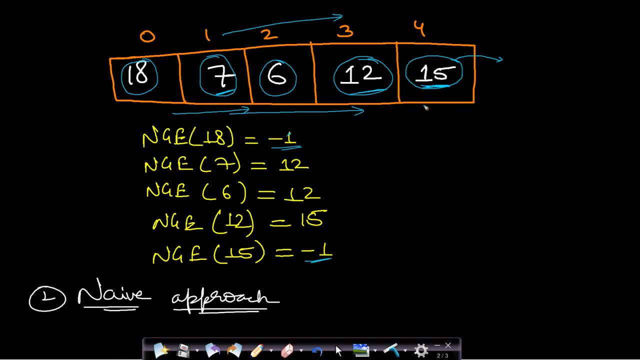 it will always be minus 1, so i hope you understood the problem now. now, how can we solve this? actually, what we can do is for a simple solution: we can pick one element and we can iterate through all the elements to the right hand side and we search for an element which is greater than this current. 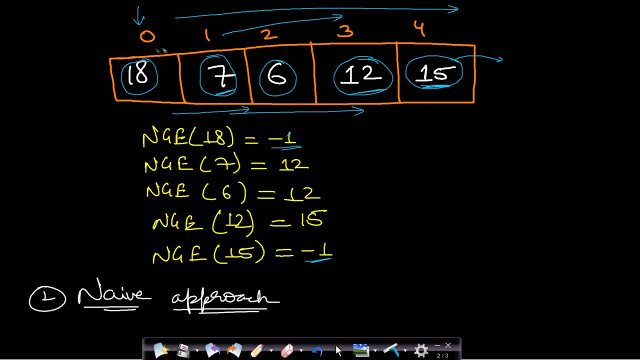 element. so as soon as we find an element which is greater than the current element, then we stop there and we just copy it in our next greater element. so this is the naive or the simple approach, but this will take order of n square time. if your array is in descending order, let's say it: 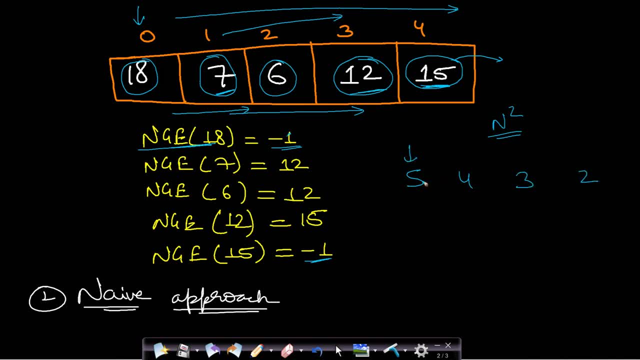 is 5, 4, 3, 2, then in this case you can see that for an element 5, you will keep searching for all the elements to the right hand side till you find an element which is greater than 5. but there are no such elements, so you will have to. 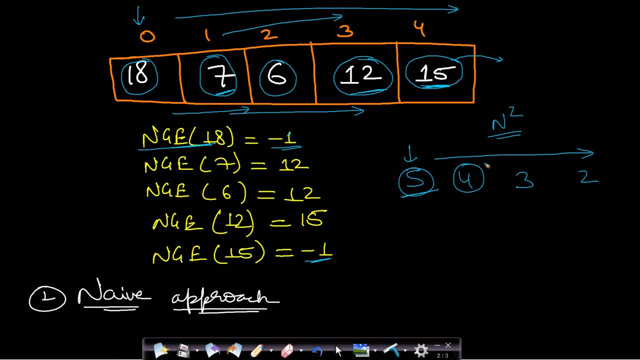 traverse for all the elements. similarly, for this 4, you will have to traverse for all the elements lying to the right hand side of 4 and adding up these computations will be order of n square. so let us look at a better solution which will solve this problem. in this case we will take an array. 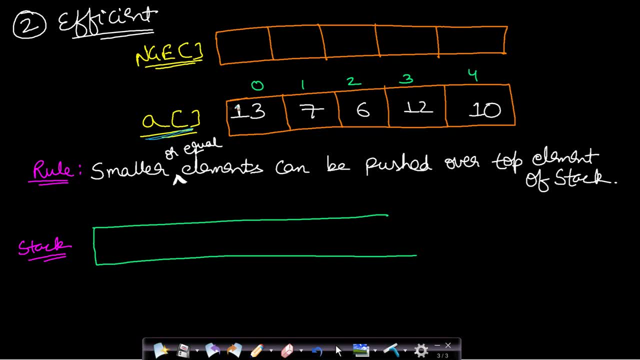 of five elements and we want to find the next greater element of each element of this array and therefore we have taken this next greater element array, so this will be storing the corresponding next greater elements. okay, now we will make you use of a stack. what will be the rule for pushing elements to the stack? the smaller or equal elements? 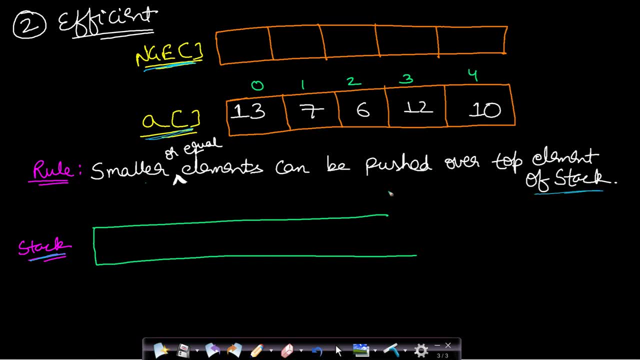 can be pushed over the top element of the stack. so let us solve this problem and you will get it eventually. so what will happen is the first element, which is 13, will be pushed into the stack. so we will push indices instead of the values. so we will push 0, which is the index of the first. 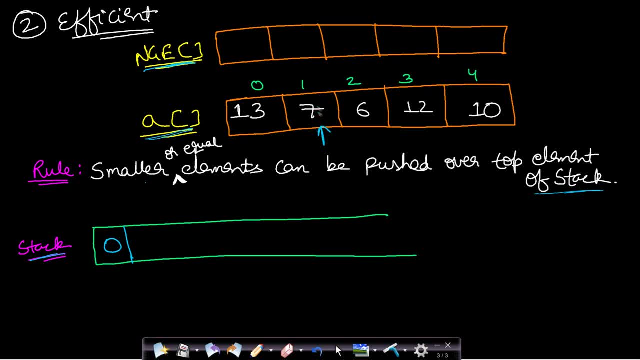 element. now we will iterate from the second element. now, since this second element, 7, is lower than 13, it will be pushed into the stack. therefore, it can be pushed on top of the stack, so we will push its index, since this was our rule for pushing. any smaller or equal element can be pushed over the 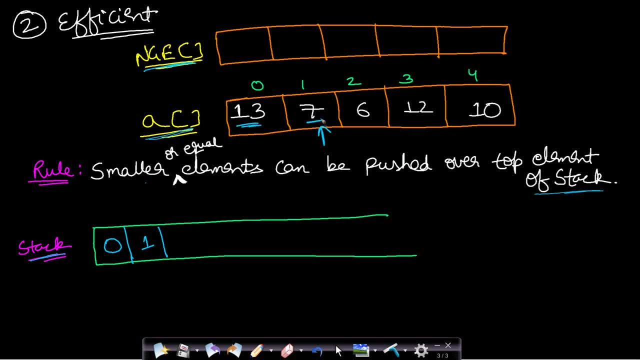 top of the stack. okay, so the top of the stack is 13 and this current element, 7, is actually lower than 13 and therefore it can be pushed over this 13. okay, so this is how we have pushed this element in the stack. now we move on to the next element. this is 6.. 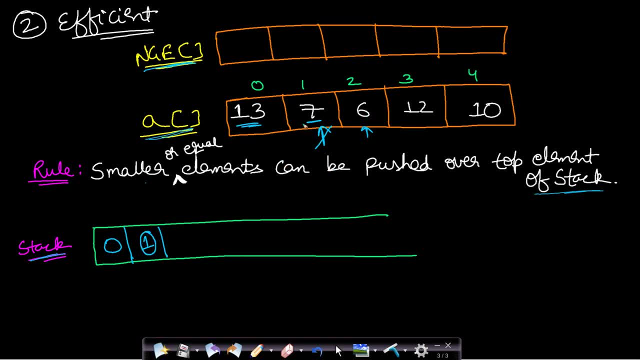 lower than the top of the stack. top of the stack is having a value 7. this is just. the index value is 7.. now 7 is greater than 6, so the current element is lower. therefore, it can be pushed. so we will push this index 2.. now we will move on to the next element. the next element is 12.. now, 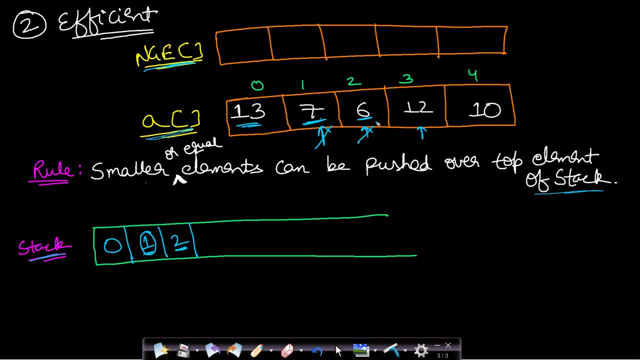 you can see that the top of the stack is index 2 and it has value 6, so 6 is actually lower than the current element. therefore, you can see that we have found the next greater element to the top of the stack. so this top of the stack is having value 6 and the next greater element is the current. 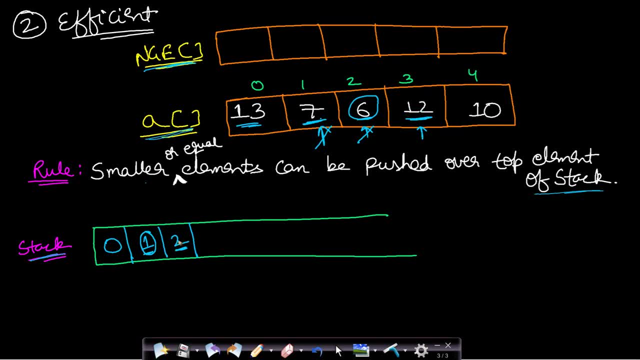 element. therefore, we will not push this current element. instead, we will pop this top of the stack, which is 2, and when we pop it, then, in place of this index, in next greater element array, we will put the current element, which is 12.. you can also store the index of this 12, but i will. 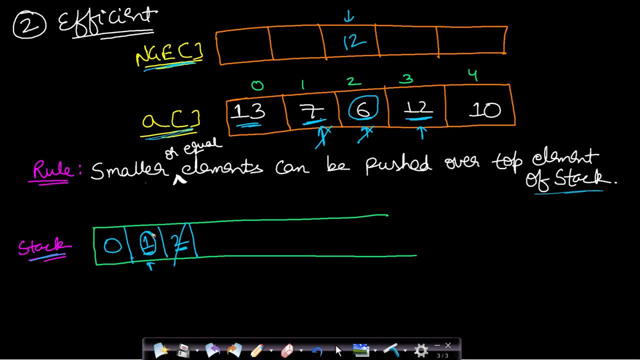 store the value here. now we will check for the next element, which is the top of the stack. its index is 1.. now you can see that 7 is also lower than the current element 12.. so we will pop this current element and then in its index, that is, index 1, we will put the current element, since we have found 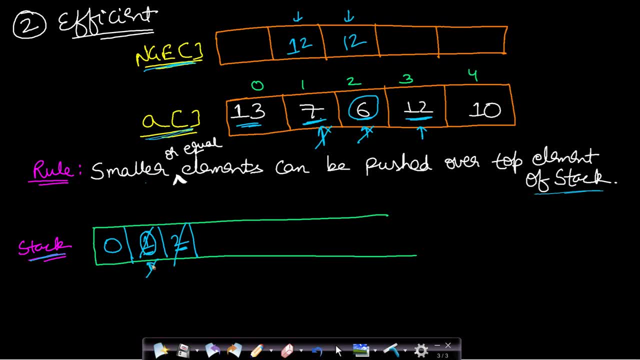 that the current element is greater than the top of the stack. now we will again move to the new top, which is index 0. index 0 is having value 13.. now, 13 is greater than the current element, 12, so we will not pop it and since our rule says that smaller or equal elements can be pushed over the